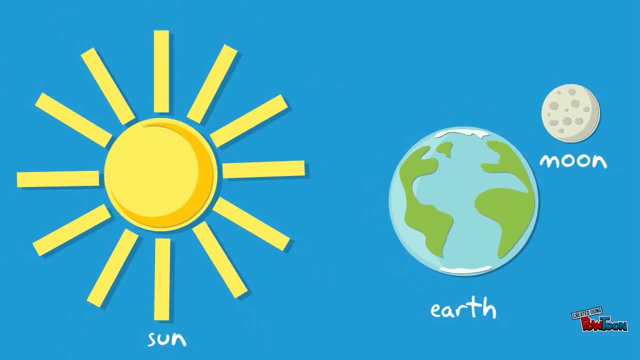 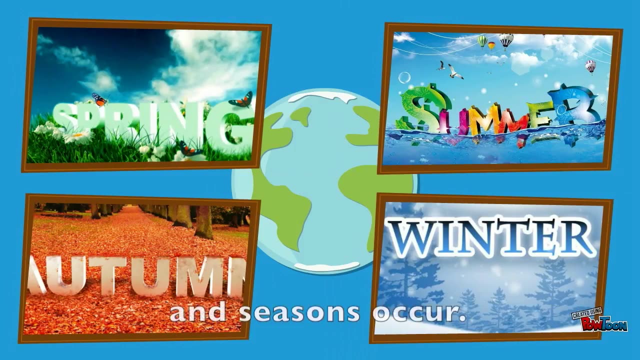 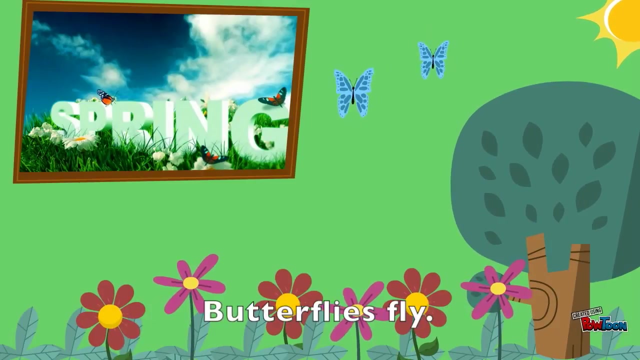 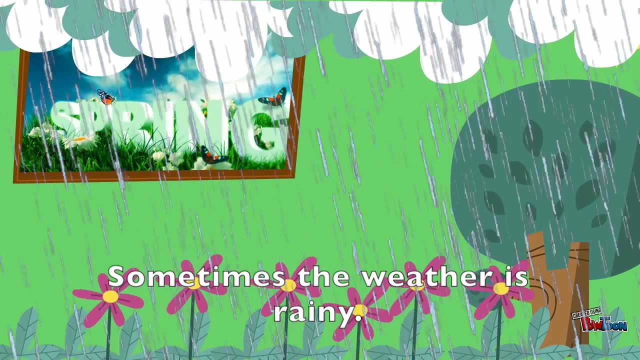 The sun, the earth, the moon. The moon spins around the earth, The earth spins around the sun And seasons occur: Spring, summer, autumn, winter. In spring, leaves are green, Flowers blossom, The weather is warm, Butterflies fly, Birds sing. Sometimes the weather is cloudy, Sometimes the weather is rainy. Open your umbrella. 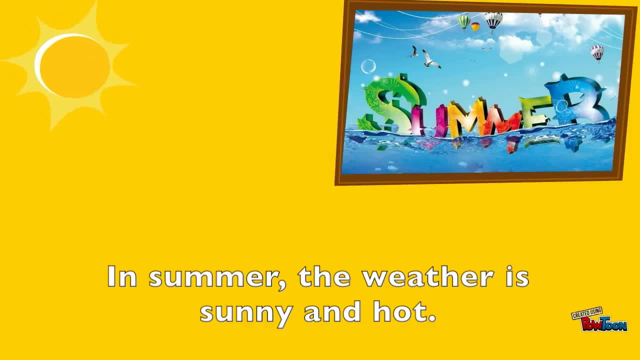 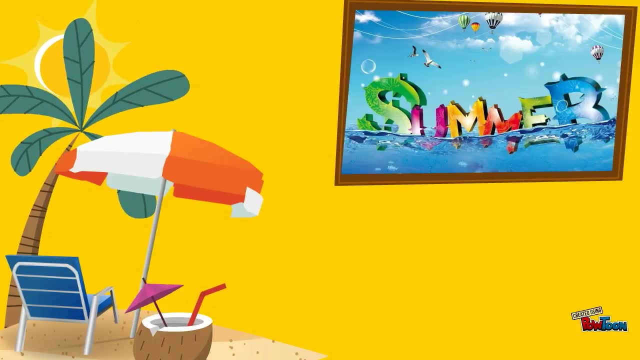 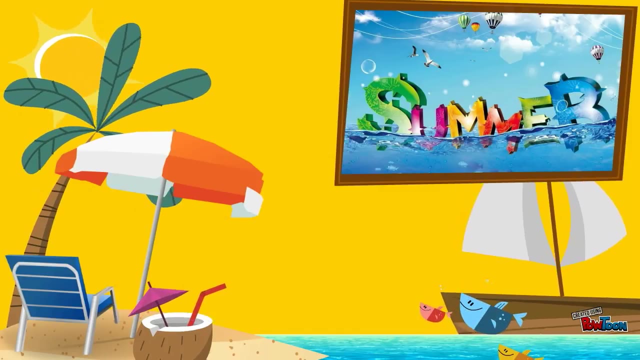 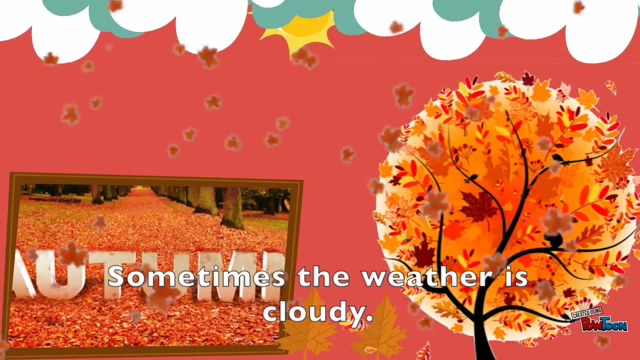 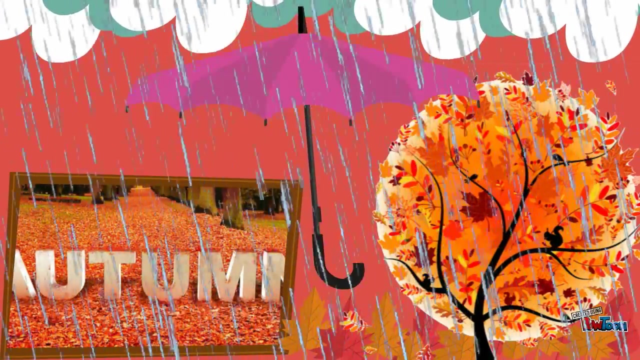 In summer, the weather is sunny and hot. You can go to the beach, You can drink cold juice, You can swim in the sea, You can sail on a sailboat. In autumn, the weather is cool. Leaves are red and brown, Sometimes the weather is cloudy, Sometimes the weather is rainy. Open your umbrella. 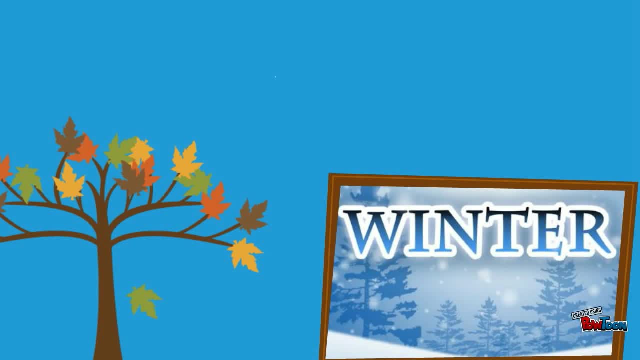 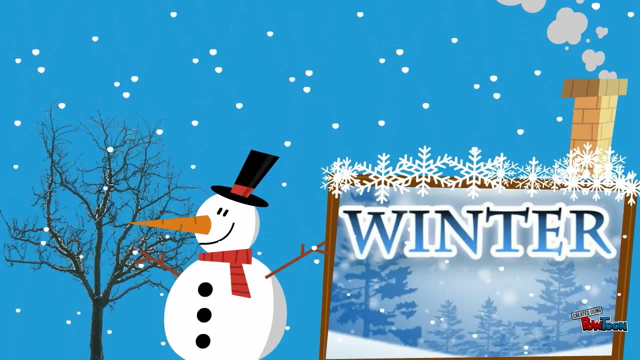 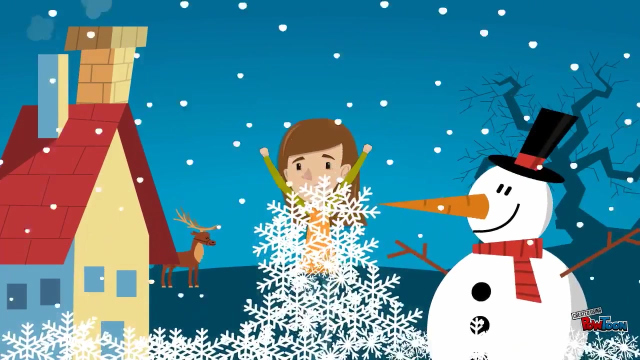 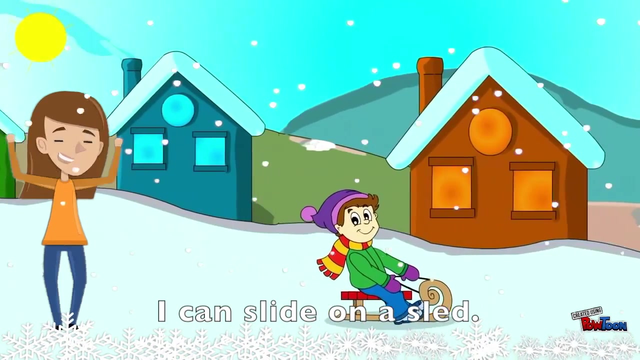 In winter the weather is cold, Sometimes the weather is snowy. Open your umbrella, You can make a snowman. What's your favorite season? My favorite season is winter, Because in winter I can slide on a sled, I can ski. 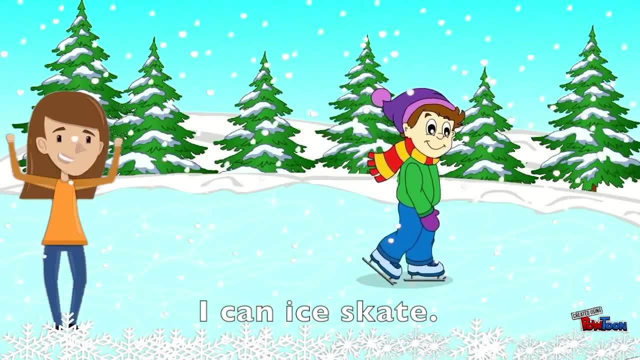 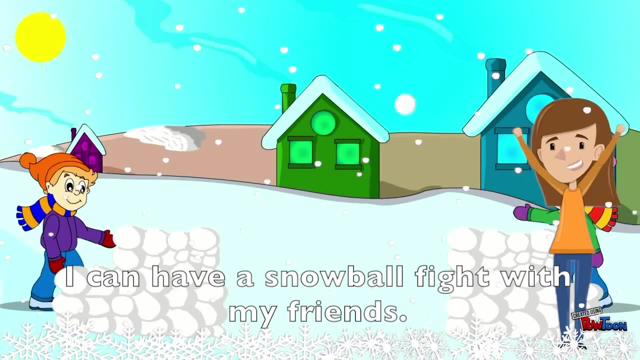 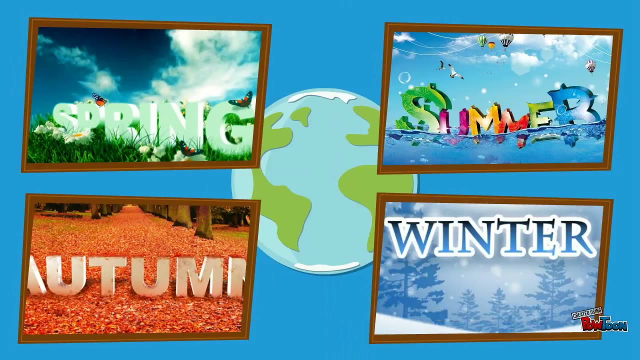 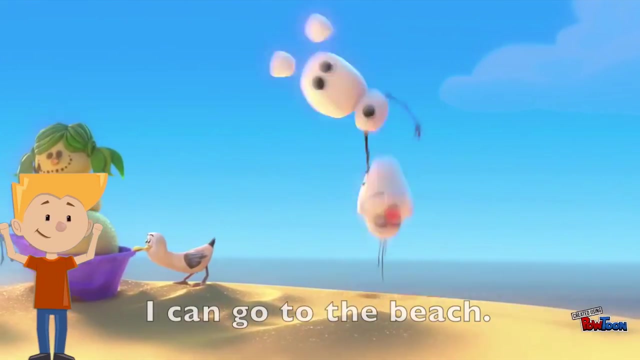 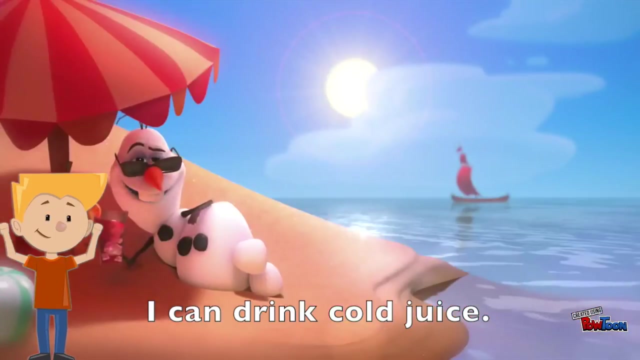 I can ice skate, I can make a snowman, I can have a snowball fight with my friends. What's your favorite season? My favorite season is summer, Because in summer I can go to the beach. I can drink cold juice. 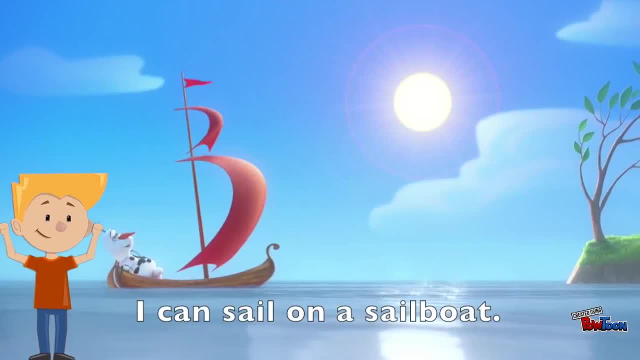 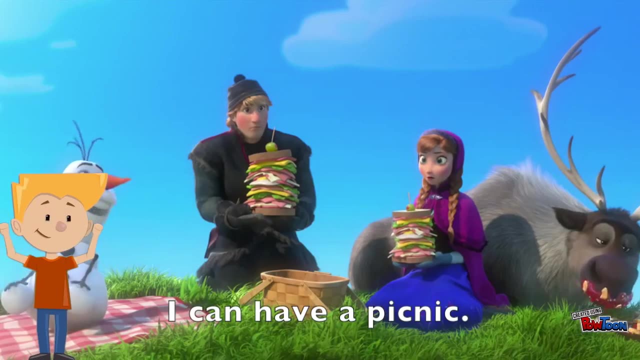 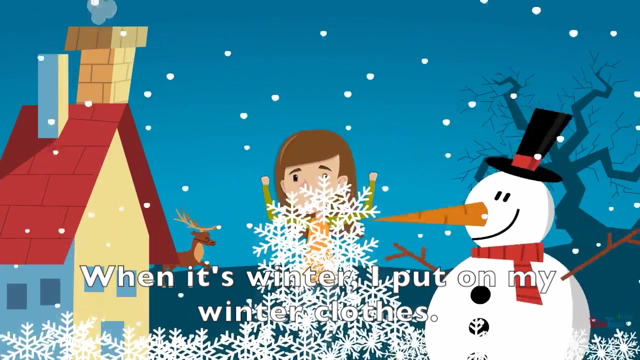 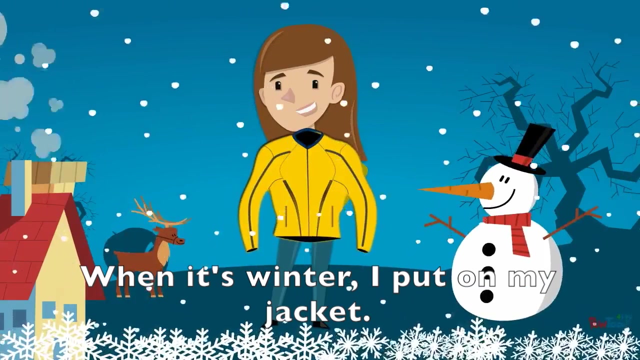 i can sunbathe. i can sail on a sailboat, i can swim, i can have a picnic. when it's winter, i put on my winter clothes. when it's winter, i put on my sweater. when it's winter, i put on my jacket. when it's winter, i put on my coat.